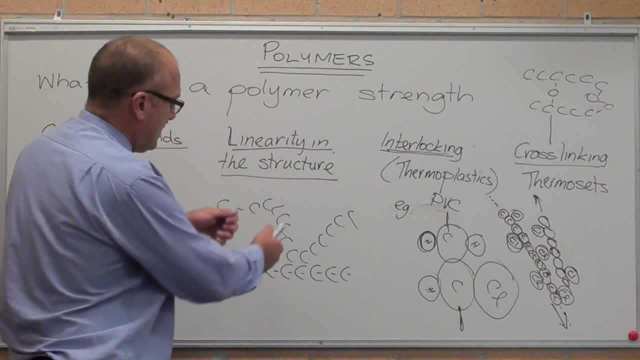 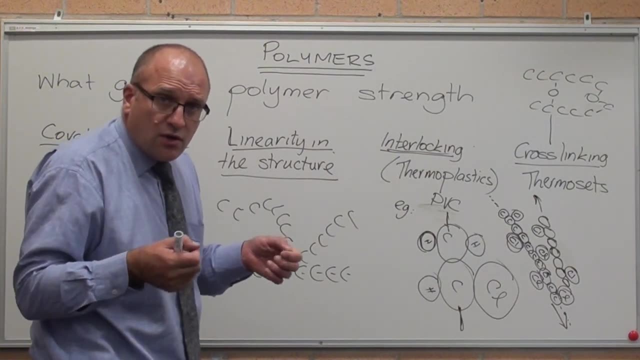 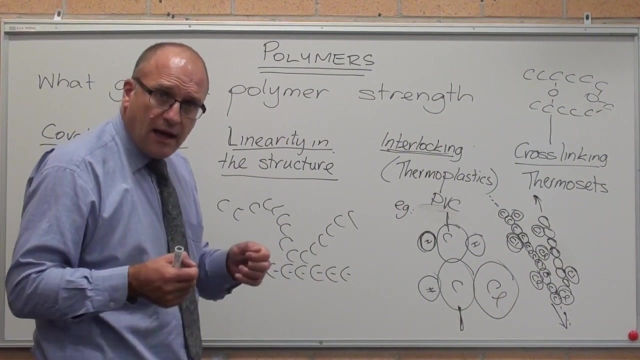 If, however, the carbon bonds are flexible and weak, you need to spend a lot of time on it. You need a lot of force straightening them out. Grab a bit of glad wrap. try and pull it out. You'll notice just before it snaps it turns white. The white is where the chains are starting to turn linear and block light coming through the glad wrap. 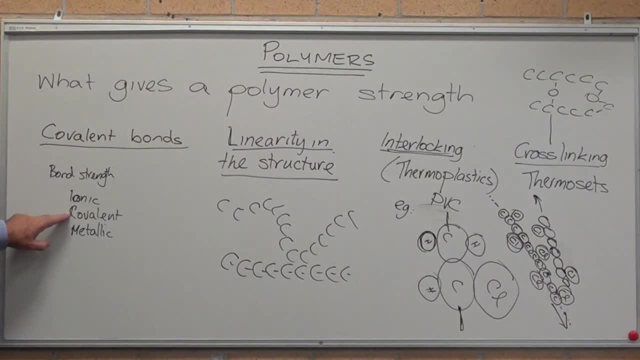 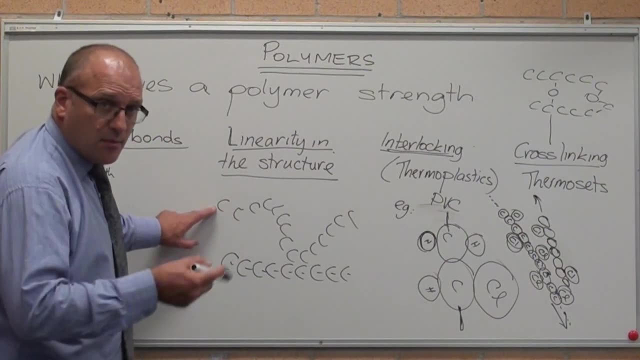 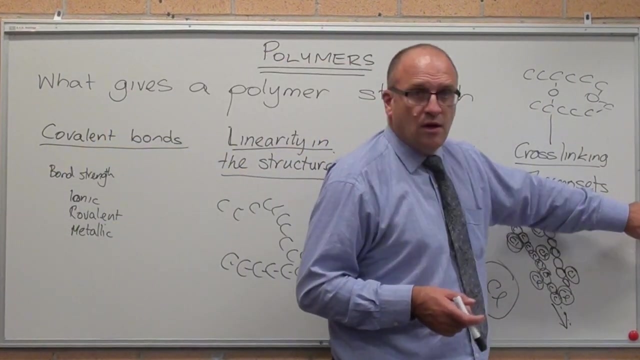 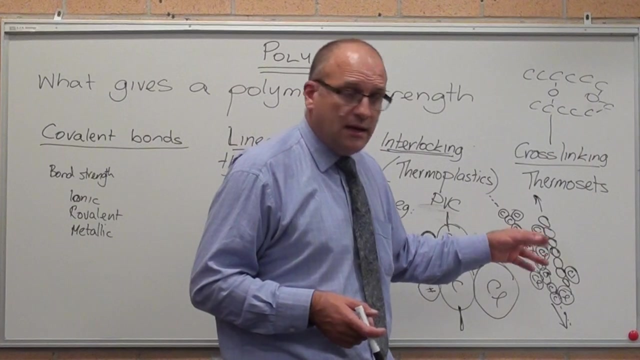 So polymers are strong because of the strength of their inherent bonds. They're strong if they have a linear structure, not a random non-linear structure. They're strong when they interlock, like this one: polyvinyl chloride. This, I hope it's in the view, this electrical conduit here is polyvinyl chloride. 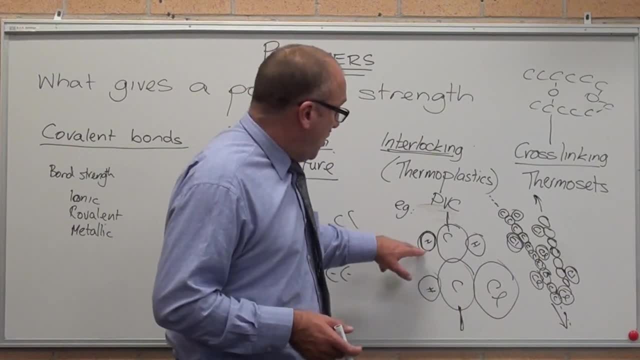 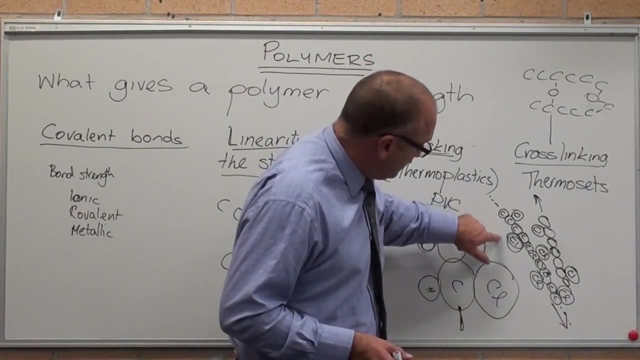 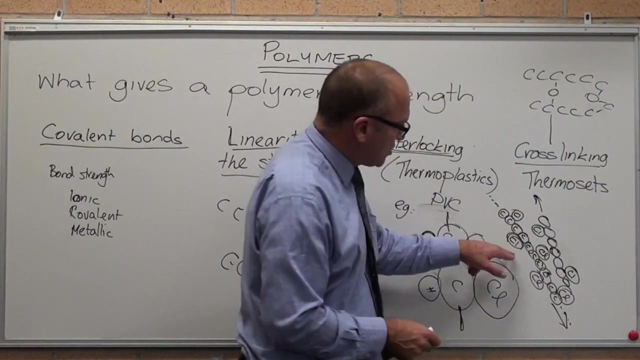 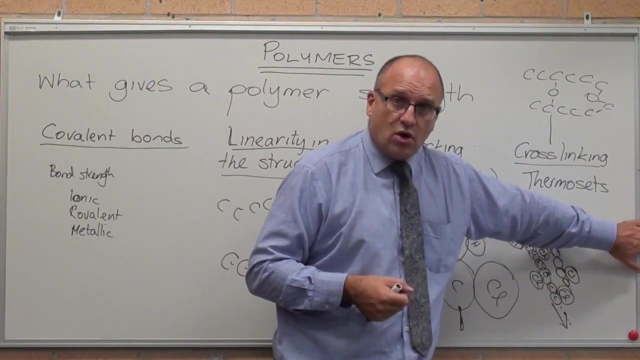 Carbon, carbon- I've drawn these about the scale. Hydrogen and chlorine is a little bit bigger than the carbon. So what happens if that's one chain of polyvinyl chloride and there's another chain? The chlorine atoms hanging out the side of the chain catch each other and stop it from moving, which is why this electrical conduit is hard, as in not flexible. 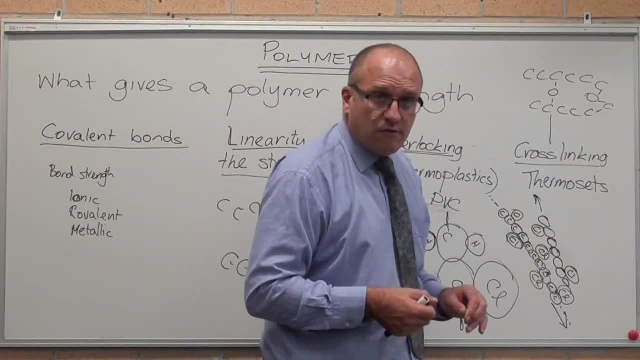 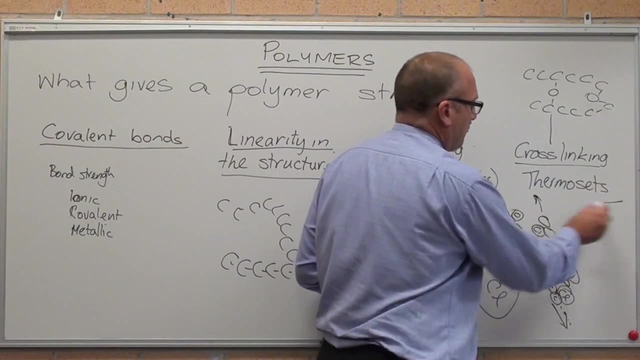 That's a better word than hard. The electrical conduit is not flexible because those chains lock together and stop it from moving. Of course, thermosets- as you know- I've drawn it up above The carbon chains- are linked together with a cross-section. 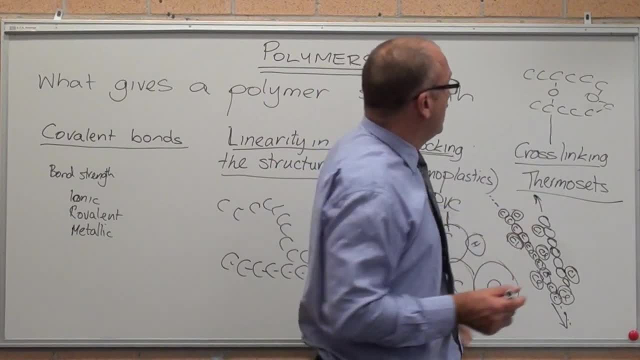 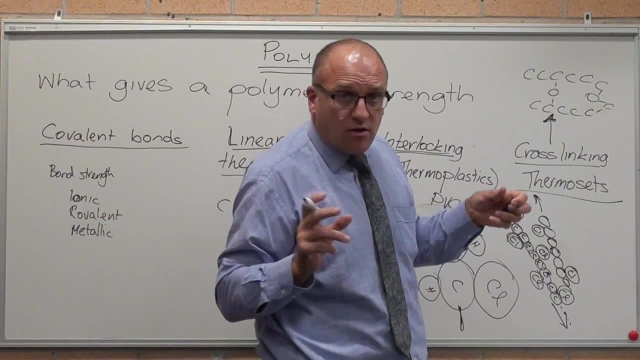 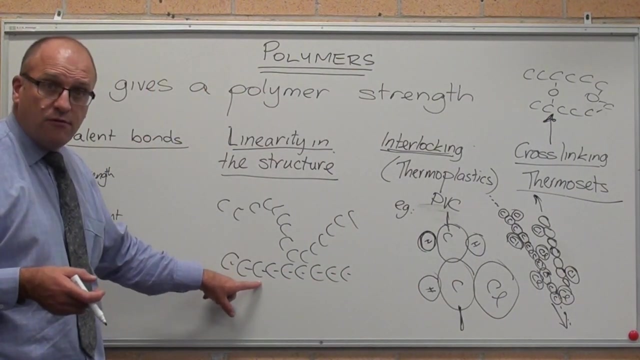 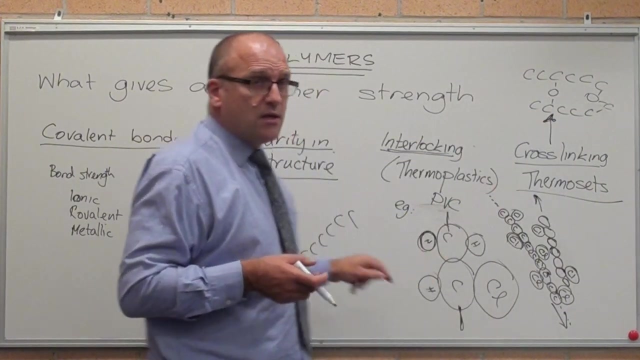 They're a cross-linking agent, usually oxygen or sulphur, So they cannot move because the entire block of polymer is physically fused together. so the atomic chains can't move. If the atomic chains can't move, high strength. If the blocks are locked together, it also gives you high strength. 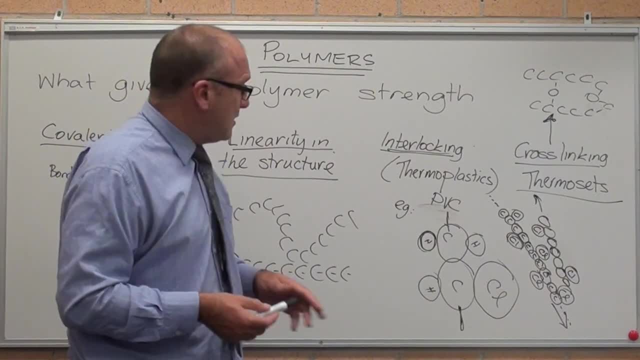 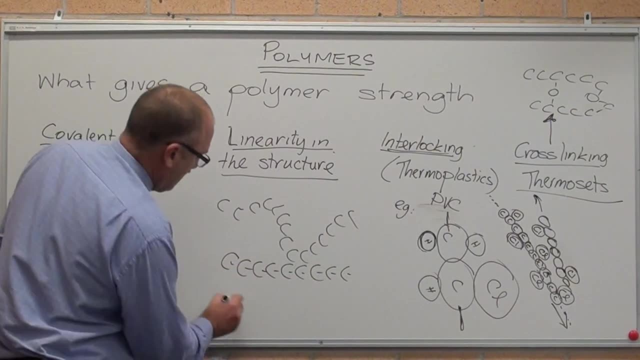 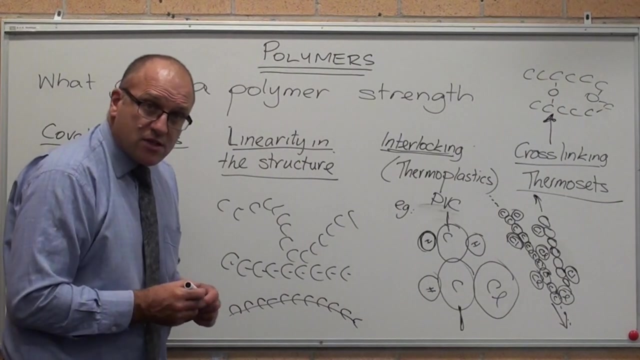 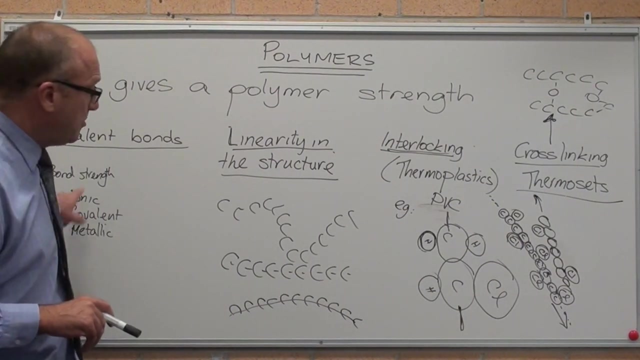 So that is where polymers get their strength from. They get their flexibility from the flux. In fact, the structure is not usually linear. Even carbon fibre. you can put a slight bend in the carbon chain like that and still get flexibility. Polymers are flexible because the covalent bond allows some rotation and movement.